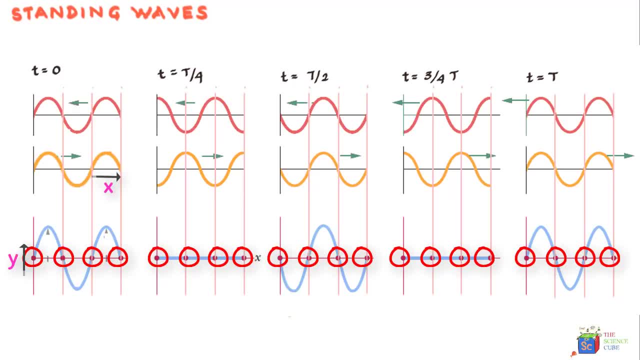 are taking us to where? what conditions are there? what judgements? what лучше? what is the trueness here to try to mention to't take? how is it? why is it so healthy to dunno and s'? 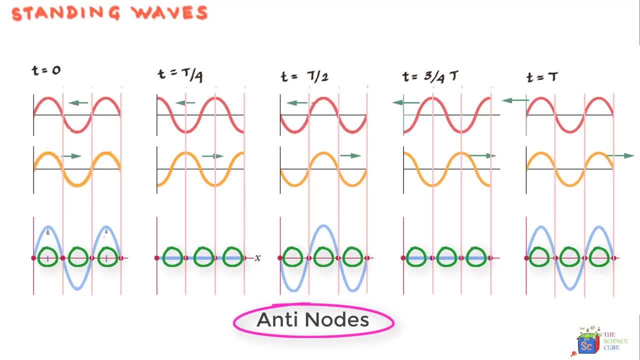 t. so these wave patterns are what we call standing waves. and you might ask why, why these should be called standing waves? because they look quite like, visually at, least, any wave we have dealt with so far. well, we say that these are standing waves because the wave pattern does not move to left. 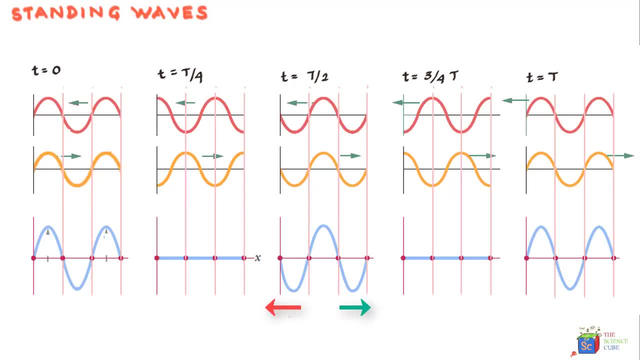 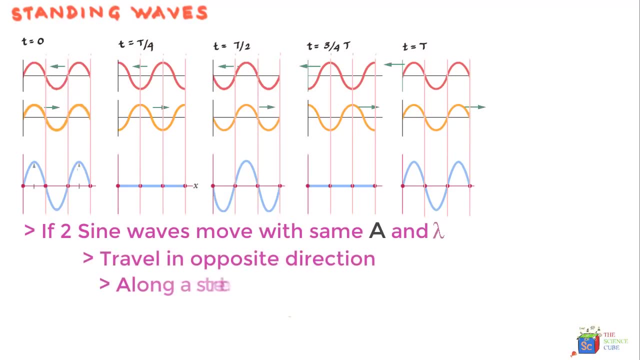 or right? so what we can say in a summary statement is that if two sinusoidal waves having the same amplitude and wavelength travel in opposite directions along a straight string, they can interfere to produce a standing wave which does not move like a traveling wave. so let us take 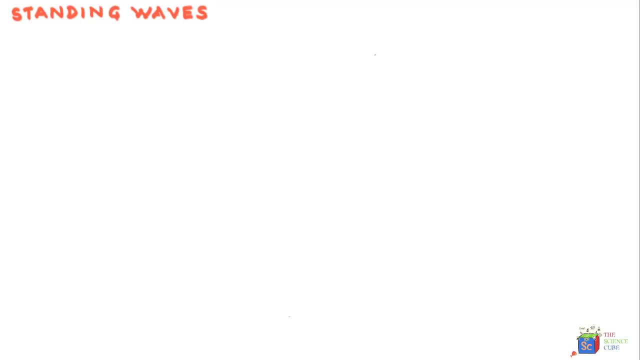 two waves of the equations: uh. 1y1 is equal to a sine kx minus omega t, which obviously is moving in the positive x direction, and the second wave is y2, y2. y2- y2 is equal to a sine kx plus omega t, which obviously is moving in the negative x direction. 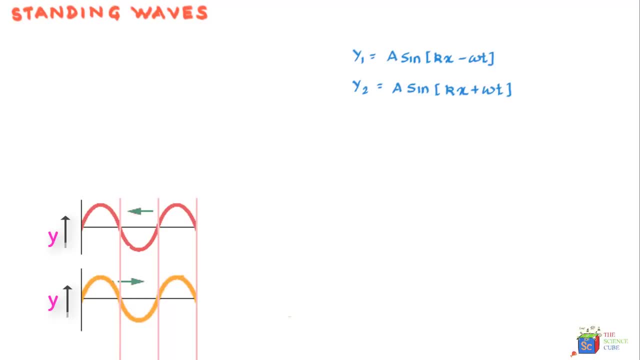 well, before we move ahead, i'd like to make a clarification around a question i have received from some of you, and the question is that when we started the chapter, we took a cos kx minus omega t as an equation to represent a waveform. and now, in the subsequent lessons we are taking, 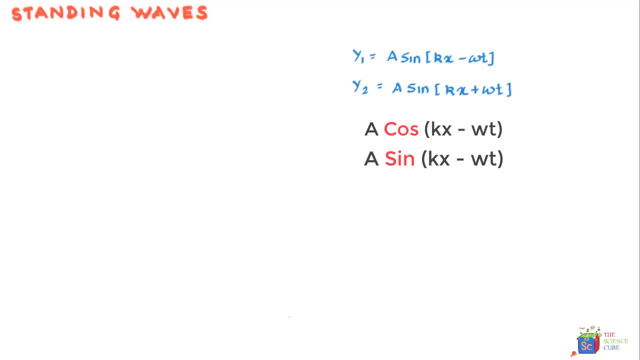 a sine omega t minus kx to represent a traveling wave. so the question is: can we take sine and cos both to represent traveling waves? so if you consider a waveform represented by a general equation like y is equal to r kx plus minus omega t, where r represents any function, cos or sine function being two of them. 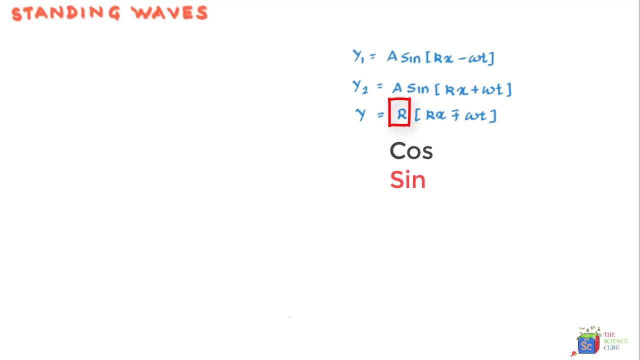 then it can be termed as a traveling wave. what is important is that this function should have a combination of x and t in the form kx minus omega t. if this combination is available, it'll be called a traveling wave. so, in short, as long as kx minus omega t expression appears on the right hand side. 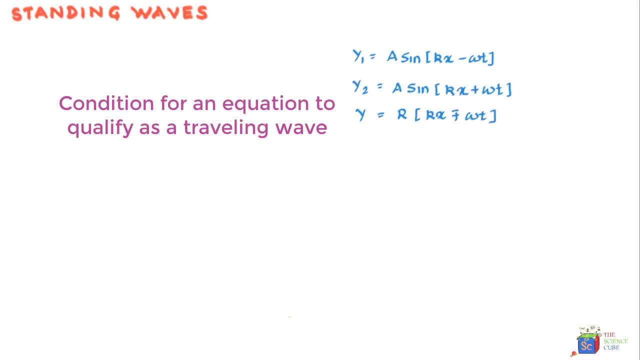 the wave qualifies as a traveling wave, and we can have sine or cos for r, both can define it as a traveling sine wave. so with this understanding, let us move ahead. and if we combine these two waves, that is y1 plus y2, what we get is a resultant wave. and let's write the equation of that resultant wave. 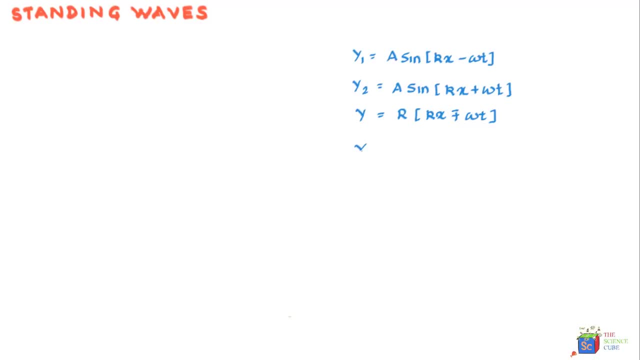 and we'll call that the displacement of that resultant wave as capital y is equal to y1 plus y2, which in turn is equal to a sine kx minus omega t plus a sine kx plus omega t. so in a way, we are adding up two waves moving in opposite direction. 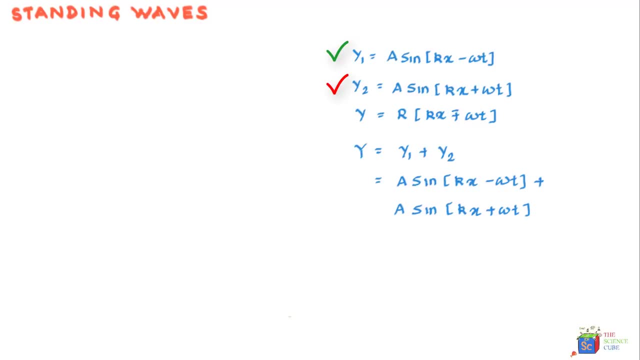 one in the positive x direction and the other in negative x direction, and if you do a bit of trigonometric jugglery around this, what you get is: y is equal to 2a, sin kx times cos, omega t, and, from a earlier understanding of what is going to be the incident of a moving wave, that is same for surrounding waves. 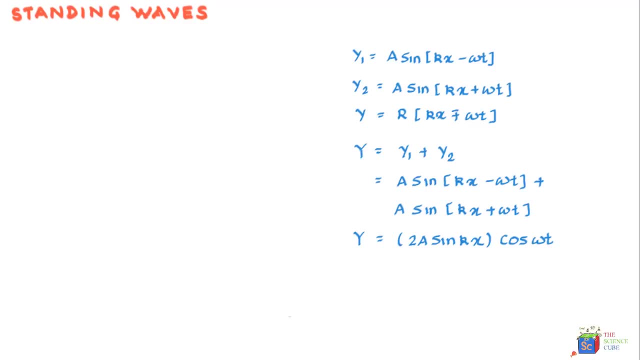 understanding of what qualifies as a traveling wave, we can clearly see that this equation definitely does not have the expression kx plus or minus Omega T, and therefore is not a traveling wave. what it actually represents is a standing wave and since it is a standing wave, unlike a traveling wave, it does not. 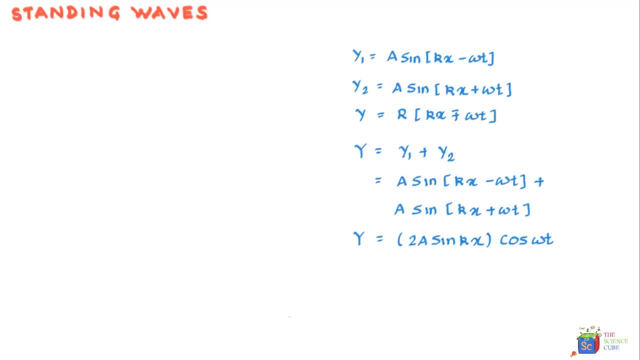 transfer energy from one end to the other. and in this equation we can see that 2a sine kx can be seen as an amplitude of the standing wave, because the max y value that you can get in this is when cos Omega T is equal to 1, but in 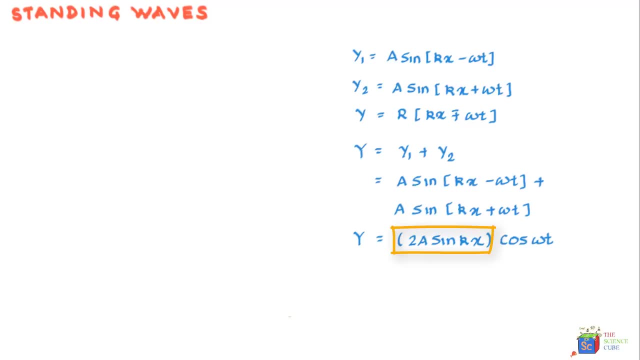 closer observation, we'll find that this amplitude is variable because it has a variable X in it. so for various X values you will have a different amplitude. and well, it seems a little strange, since normally amplitude is a constant, often represented as capital A or something like a ym. but then, if you visualize a standing wave, 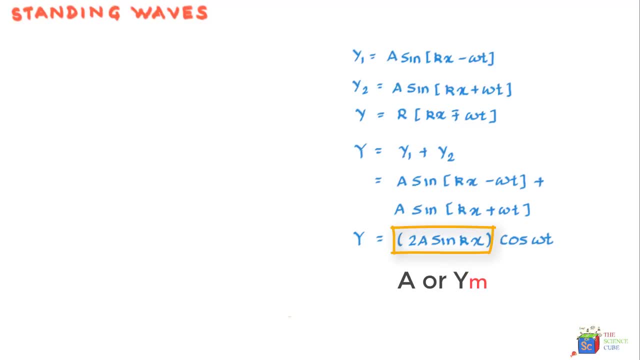 you will find that each point of the string is vibrating about y-axis and has a certain maximum y displacement or amplitude, and this is quite unlike a traveling wave where each point in the string gets an opportunity to experience amplitude, A capital A, which is, which is a maximum displacement that a traveling 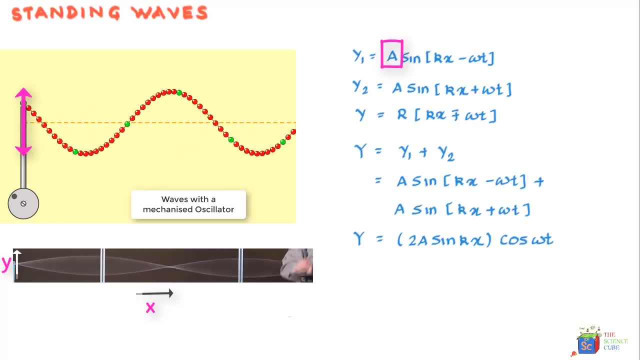 wave goes through and why each point experiences maximum amplitude in a traveling wave is because the wave is moving with a certain velocity and the wave travels. and as a wave travels, each point swings to the maximum a value periodically. so this is a unique feature of a standing wave, where the amplitude 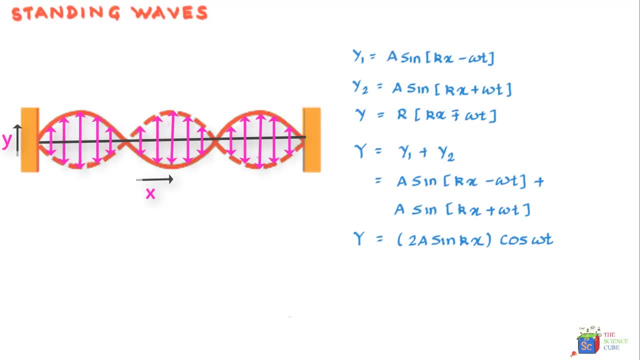 is a variable and each point on the string has its own amplitude. so we can see that the amplitude will be 0 when sine kx is equal to 0, and for this to happen kx should equal to n pi. so if we denote this amplitude as a dash, then we: 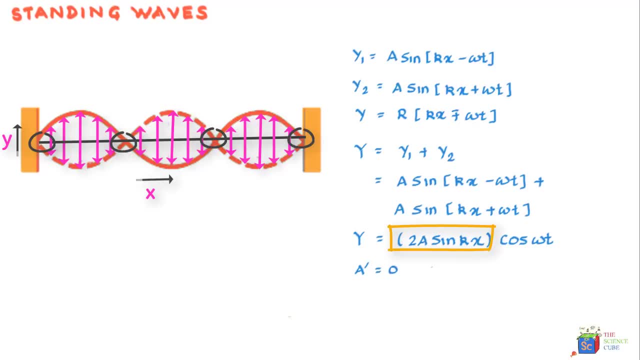 can say that a dash is equal to 0 when when sine kx is equal to 0, and for this to happen, kx should equal to a multiple of Phi. so we'll say it should be n pi where n is equal to 0, 1, 2, 3 and so on, and if you take k is equal to 2 pi upon. 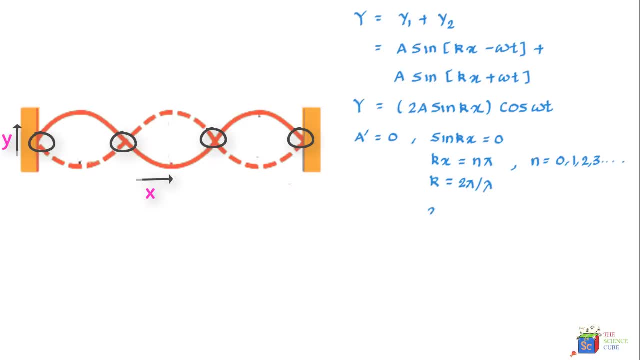 lambda, what we get is x equals n lambda upon 2.. so we've taken us from the varsity exercises with these ну. thanks for your attention. taken, this expression, k is equal to 2 pi upon lambda and substituted in this equation to get: 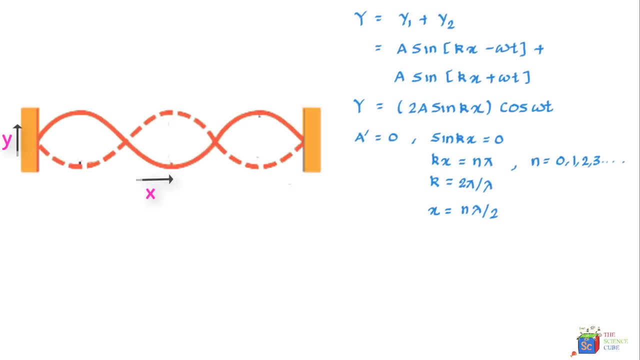 x is equal to n lambda upon 2.. So you get your nodes for all such x values where the point does not move at all. You can also see that each node is separated by lambda upon 2, as in: if you take a certain value of n and you take the consecutive value, let's say you take n as 5 and then you take. 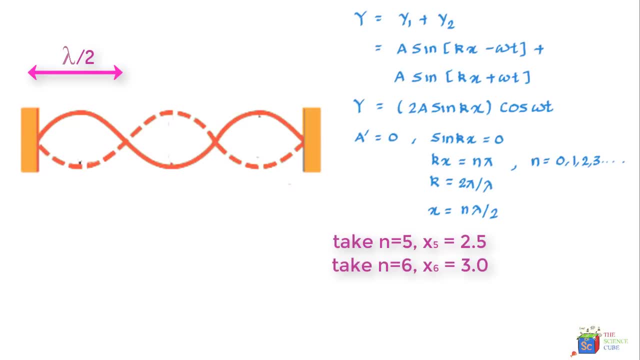 n as 6 and you substitute: n is equal to 5 here and then n is equal to 6 and you take the difference. you'll get the difference as lambda upon 2 and the amplitude will be 2a, which is the maximum amplitude possible. That is what we are saying is a dash would have a maximum amplitude which is 2a. 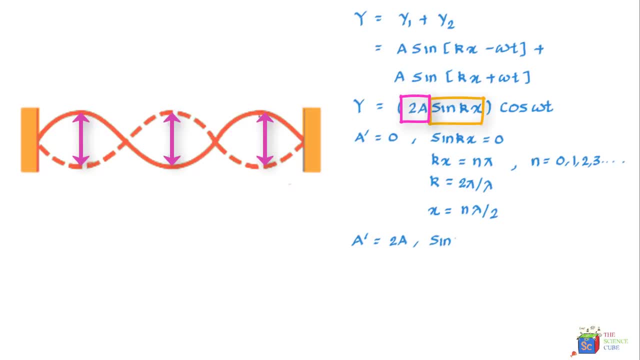 when sine kx is equal to 1 and for this to happen, kx should equal pi by 2, or 3 pi by 2, or 5 pi by 2, and so on. or we can say that kx should equal n plus 1 by 2 pi. 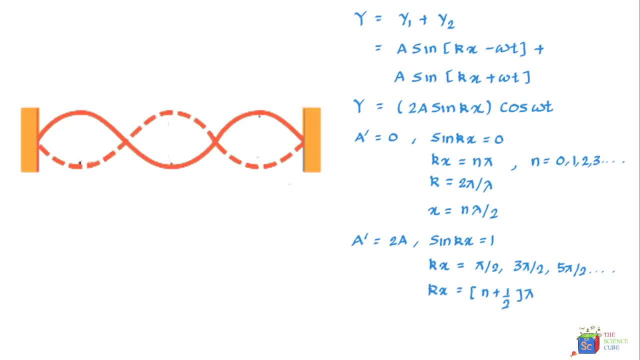 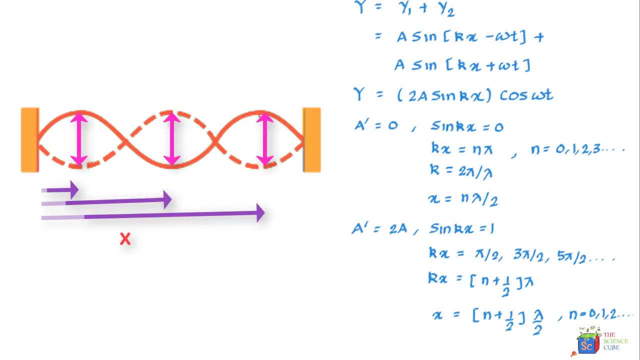 and again, if k is equal to 2 pi upon lambda, then what you get is: x is equal to n plus half lambda upon 2.. For all n values of 0,, 1,, 2 and so on. So you get your antinodes at all these x values, and here also. 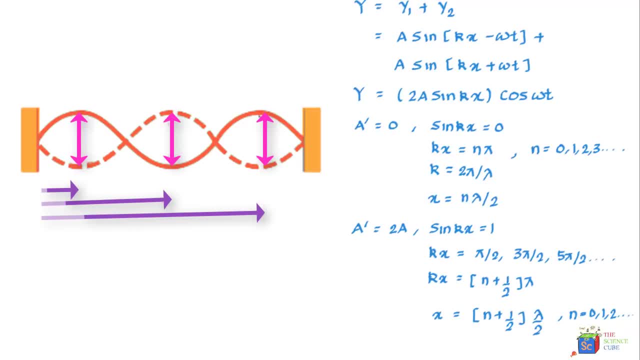 you can see that the difference between each antinode is half a wavelength. Well, you can put: n is equal to any value, say 6 and then take n is equal to 7 and then take the difference. you'll find that the difference comes to lambda upon 2.. 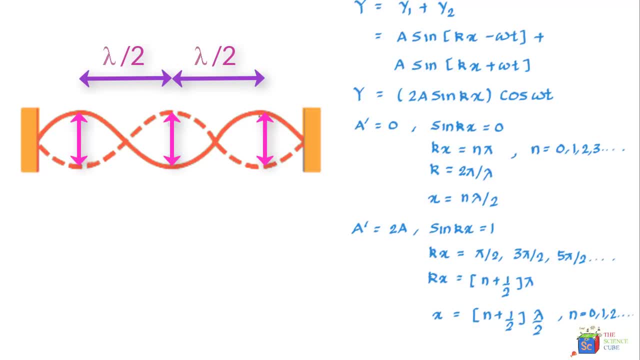 And this will be true for any two consecutive n values. So that brings us to the topic of resonance. So let's take a guitar string and stretch it between two clamps and send a set of sinusoidal waves of a certain frequency through the string in the 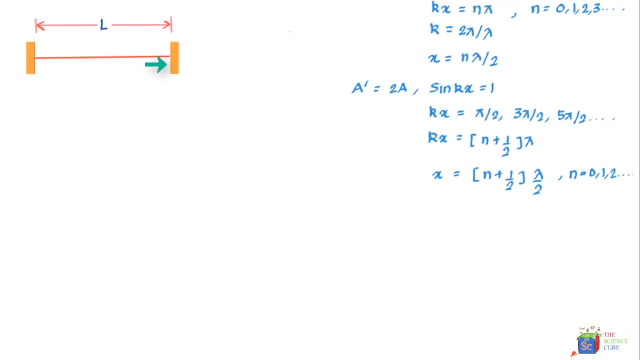 positive x direction. Then, as the first wave reaches the right end, it reflects and travels back to the left. Well, it is obvious that this reflects and travels back to the left. Well, it is obvious that this reflects and travels back to the left. Well, it is obvious that this. 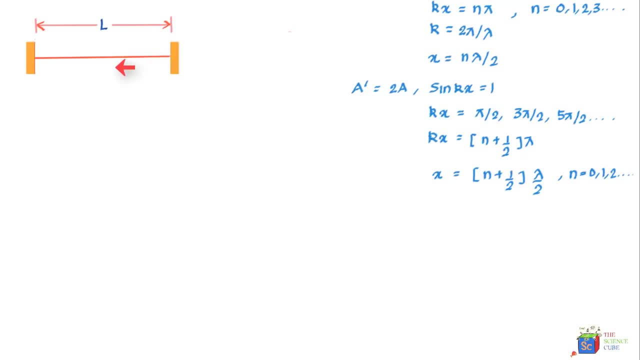 reflected wave moving to the left will overlap with the wave that is still traveling to the right, And when the reflected wave reaches the left end, it reflects again and this newly reflected wave begins to move to the right, overlapping the waves going to the left as well as the waves moving to. 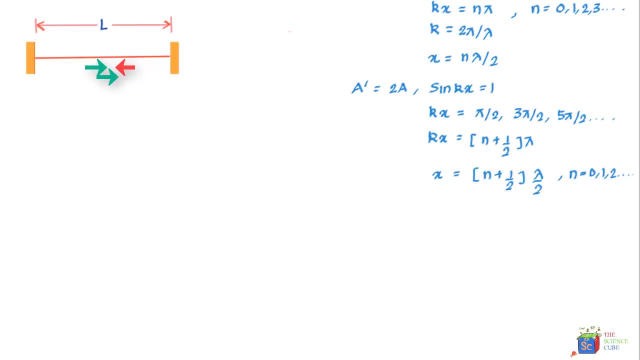 the right. And if we keep analyzing this way, we'll find that we have a bunch of overlapping traveling waves which interfere with each other, And when this happens for certain frequencies- not all frequencies- the interference produces a standing wave pattern, or you could say an oscillating pattern, with nodes and anti-nodes, like this: 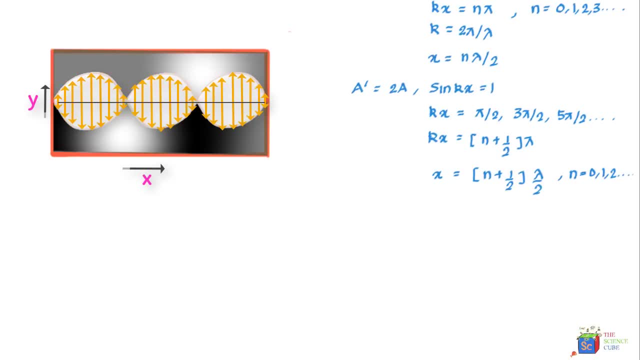 And when this happens, we say that a standing wave has been created and the chord or the string is said to be resonating at these certain frequencies that are called resonant frequencies. And if the string is oscillating at some frequency other than a resonant frequency, a standing wave will not appear. 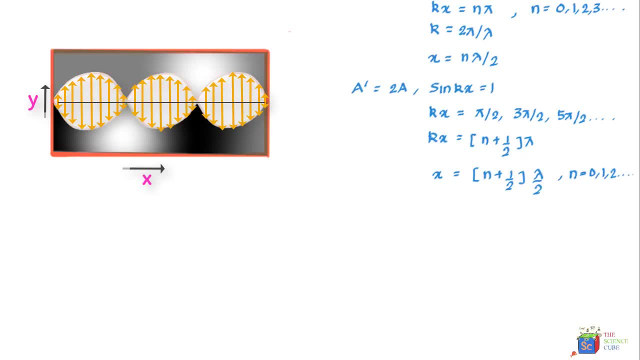 So let's take this further and see the mathematics around this. so we'll stretch a string between two clamps that are distance l apart and we'll try to find an expression for frequency that produces resonance in the string in terms of length l and velocity v of the wave. A good starting point will. 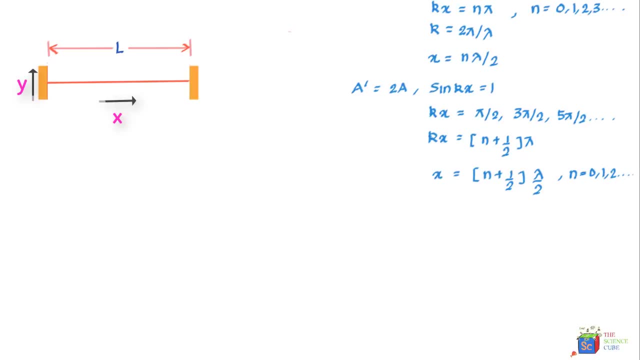 be to recognize the fact that ends of the string here are nodes, since they are stationary, and we know that this is a necessary condition for a standing wave. well, if you observe this pattern of loop formation where we have two nodes and one anti-node in between, we can say that this is a 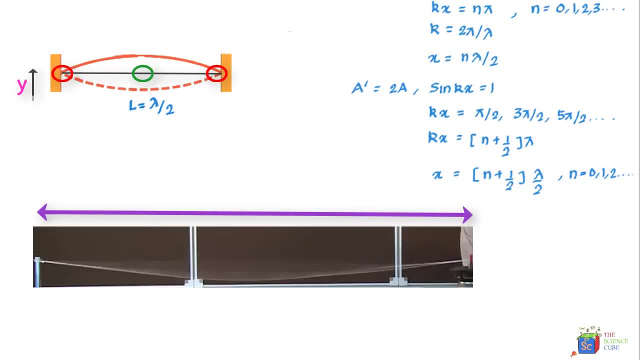 standing wave. we can also see that half a wavelength spans the entire distance, l, or the strings length. so we can say that lambda upon 2 is equal to l. we can therefore infer that if the left going and right going traveling waves have a pattern like this due to interference, 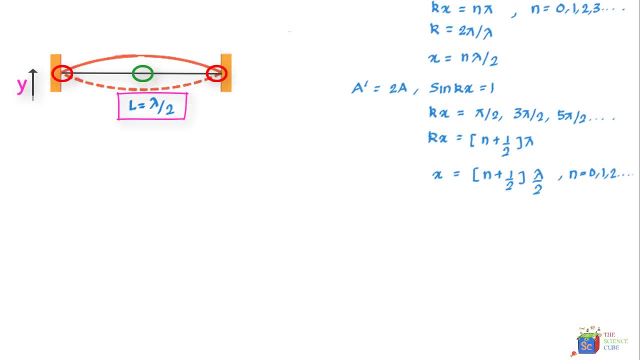 they must have a wavelength lambda equal to 2l. well, another pattern that would have nodes at n sort ofORE and X OFF, could be this: now, this one has three nodes and two anti nodes and can be named two loop pattern for waves moving in either direction. they must have a 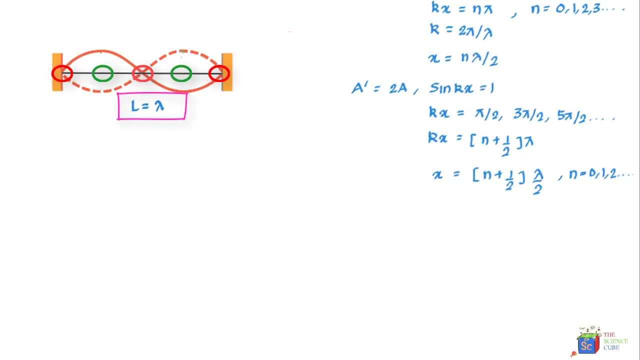 wavelength lambda equal to L. likewise, another pattern could be this: that has four nodes and three anti nodes. this, therefore, could be called a three loop pattern, and we can see that here L is equal to three by two lambda, or one and a half wavelengths. you you have this as lambda and another half a lambda, which. 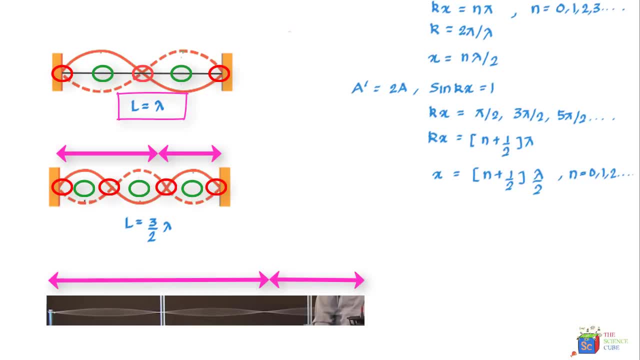 makes it one and a half lambda or three by two lambda and therefore lambda is equal to two by three L. by now you would have figured out that this can keep continuing and the patterns can have more and more loops, with more nodes and anti nodes increasing by one node at each step and an additional lambda by two. 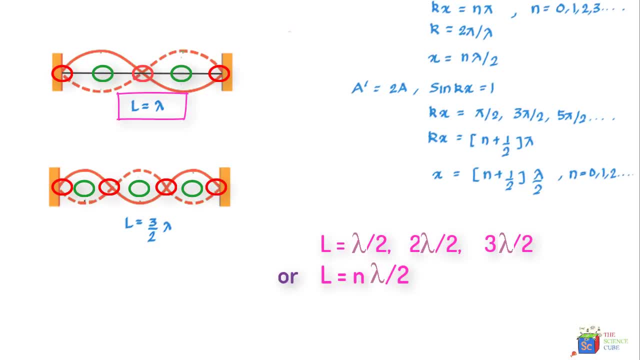 gets fitted into lambda length L, so we can set up a standing wave on a string of length L with wave that have wavelengths equal to one of the values below. that is, lambda is equal to to L upon N, for N is equal to 1, 2, 3 and so on. so let's put a subheading. 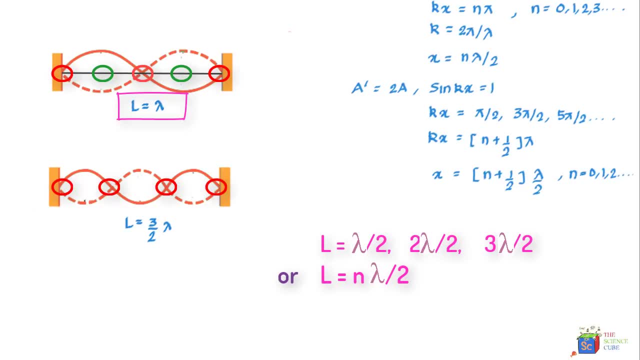 resonance over here and, as i said, we can write lambda is equal to How manyの L'-1 and R-n for each of our delta strings to 2 L upon n, where n is equal to 1, 2, 3 and so on, and the corresponding resonant. 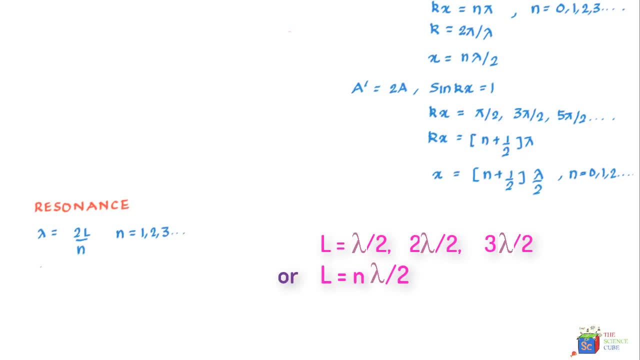 frequencies will be: F is equal to V upon lambda, and if we substitute the value of lambda in this equation, what we get is F is equal to n times V upon to it and for n is equal to. let us say 1, we get F. 1 is equal to V upon 2, L for n equal to 2. we.